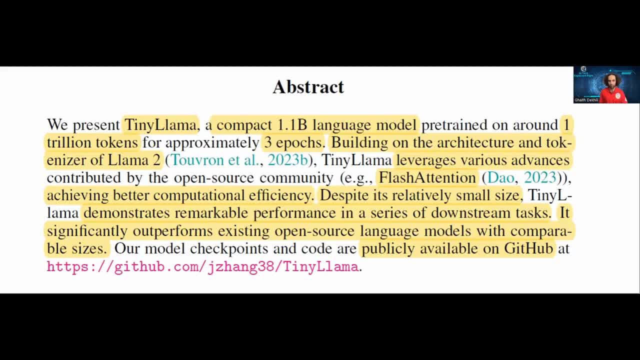 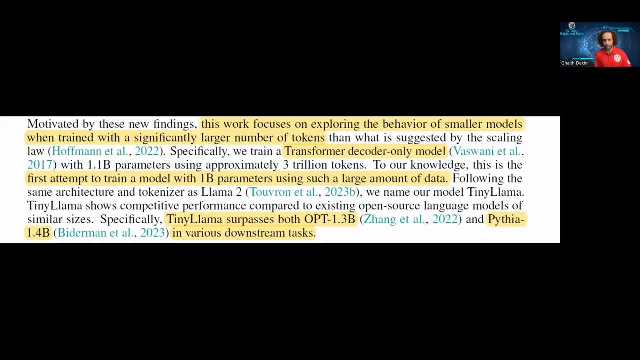 checkpoints and code are publicly available on github at the address shown here so now let's dive a little bit deeper in technical things so in their work authors focus on exploring the behavior 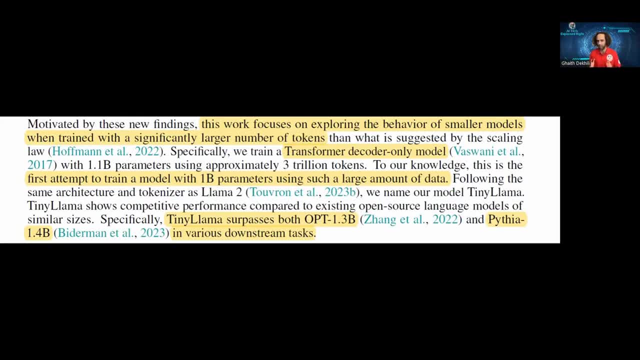 of smaller models when trained with a significantly larger number of tokens to do so they train the transformer decoder only model and this work is considered as the first time to train a model with one billion parameters and the first time to train a model with one billion parameters 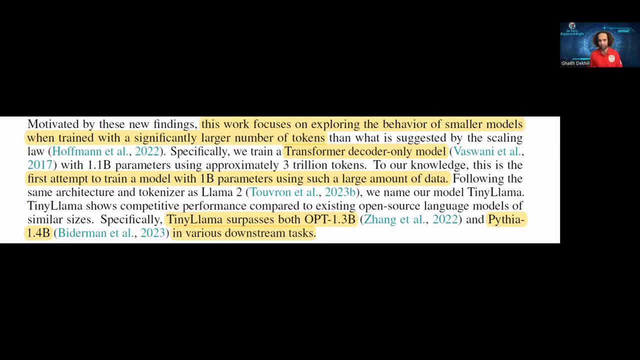 parameters using such a large amount of data in the next few minutes we will see how tiny llama 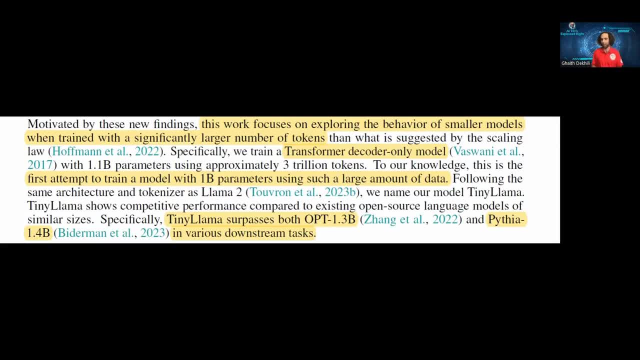 surpassed both opt 1.3 billion and python 1.4 billion parameters in various downstream tasks 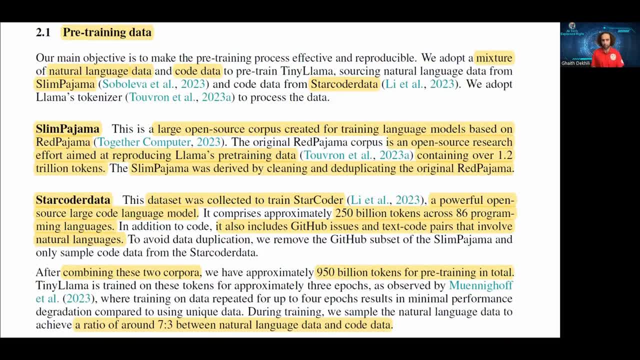 now let's talk about retraining in their work authors adopt a mixture of natural language data and code data sourcing natural language data from slim pajama and code data from starcoder data 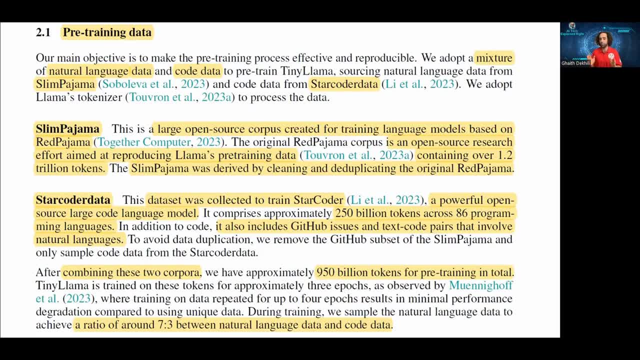 use a little bit more of context slim pajama is a large open-source corpus created for training language models based on red pajama which is an open-source research effort aimed at reproducing lamis retraining data containing over 1.2 trillion tokens 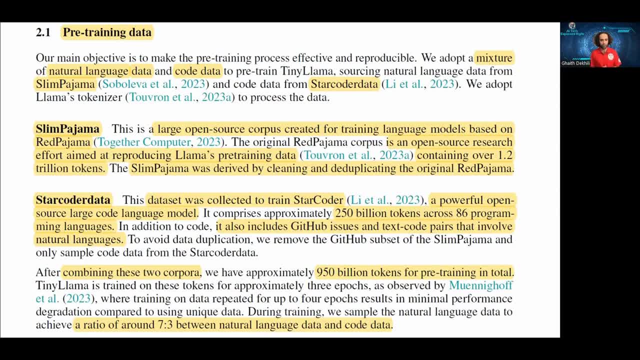 the slim pajama was derived by cleaning and duplicating the original red pajama on the other side starcoder data was collected to train start coder a powerful open source large code language model 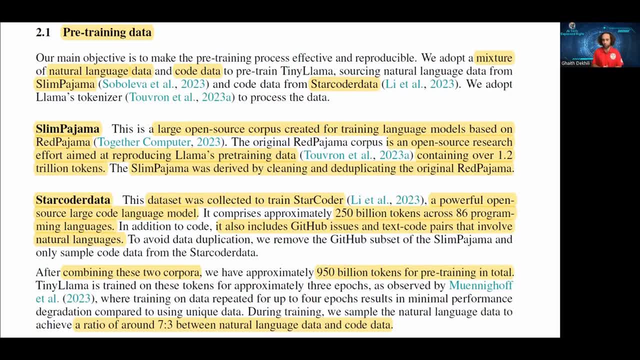 model it comprises approximately 250 billion tokens across 86 programming languages in addition to code it also includes github issues and text code pairs that involve natural language after 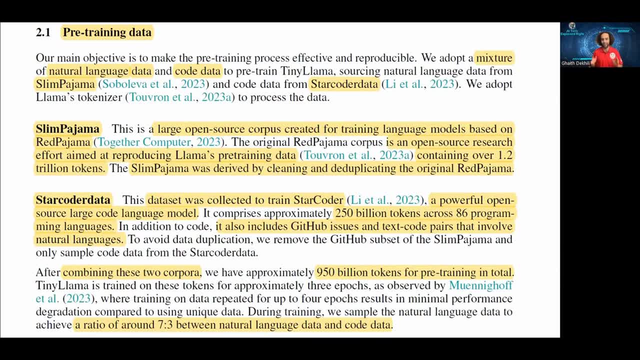 combining these two corpora authors have approximately 950 billion tokens for pre-training 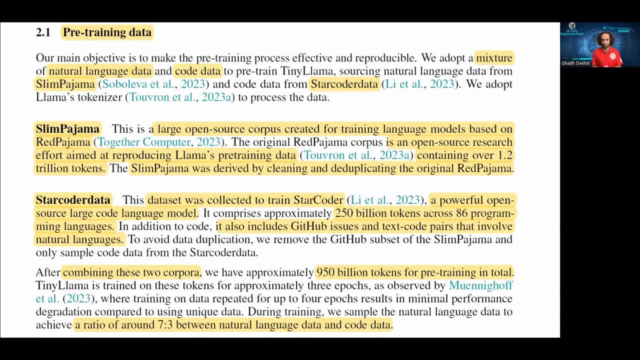 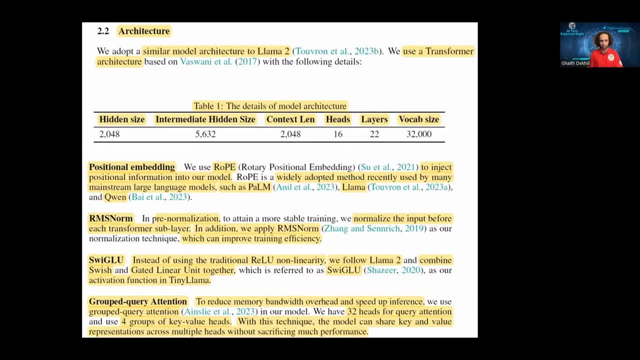 in total during training authors sample the natural language data to achieve a ratio of around 7.3 between natural language data and code data let's talk about architecture now as i already 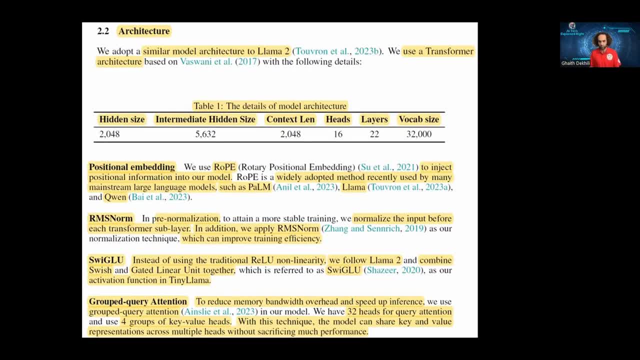 mentioned the model architecture is similar to the one used in llama 2 using a transformer architecture with the hyper parameters shown in the table one which are the hidden side the 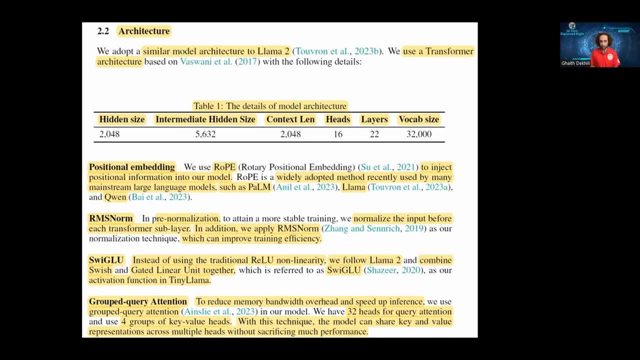 intermediate hidden size the context length number of heads number of layers and the book up size stay tuned guys with my channel by subscribing as i'm planning to create a video where i talk about the transformer architecture 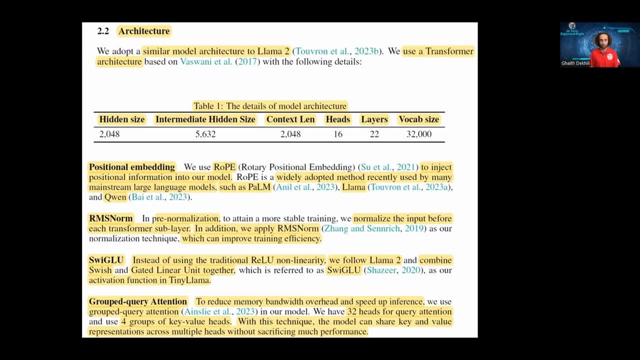 where i explain all these kind of information now in the architecture authors used rotary positional embedding to inject positional information into their model this method has been widely adopted 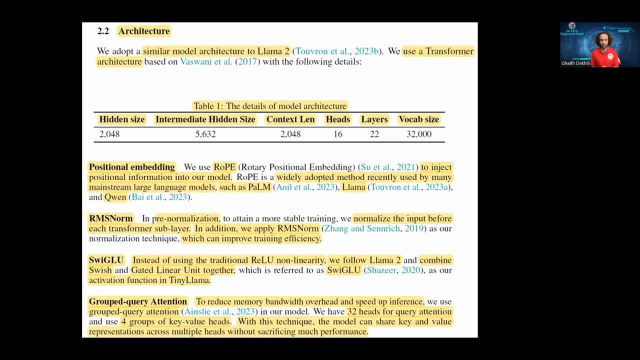 recently and has been used by many mainstream large language models such as palm lama and when authors apply rms norm as their normalization technique which can improve training efficiency this was additional to normalizing 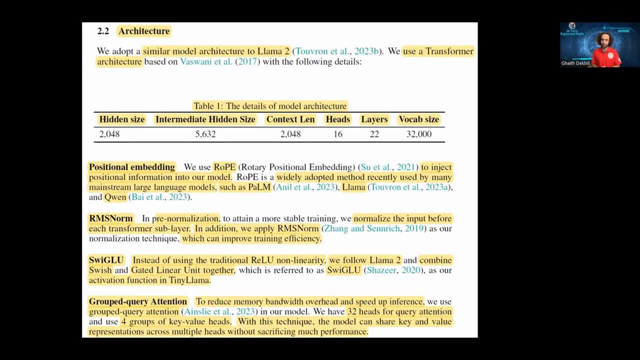 the input before each transformer sublayer in the pre-normalization phase to obtain a more stable training instead of using the traditional radio non-linearity authors follow lama 2 and combine 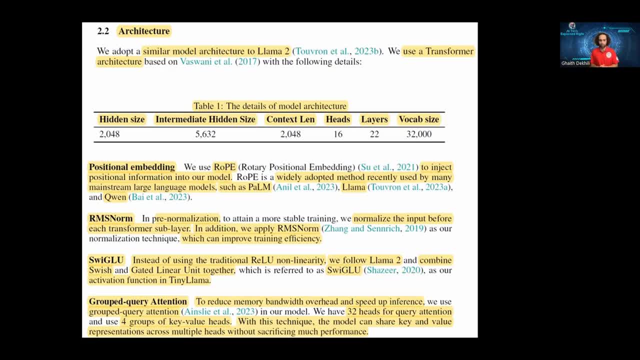 swish and glu for gated linear unit together which is referred to as swi glu and this was their activation function in tiny llama and last but not least authors used grouped query tension to reduce 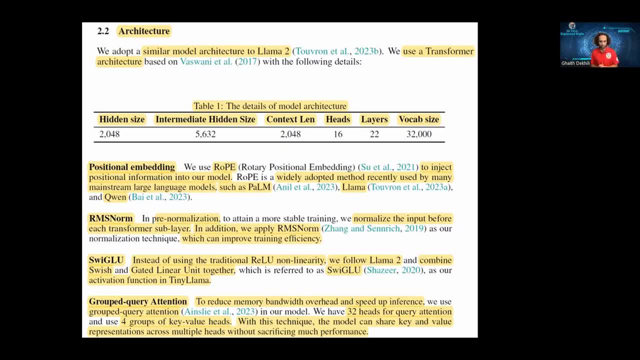 built-in memory bandwidth overhead and speed up in fibrance they have 32 heads for query attention and use four groups of key value heads with this technique the model can share key and value representation across multiple heads without sacrificing much performance now for speed 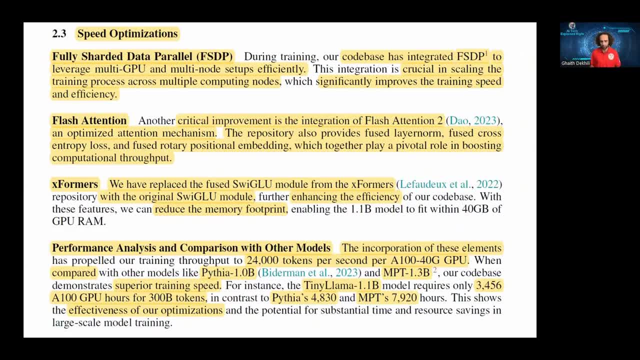 optimizations authors use techniques that have shown the effectiveness in many notable works let's start with the fully shared data parallel procedure during training. They used this technique to leverage multi-GPU and multi-node setups efficiently. This integration is crucial, guys, in scaling the training process across multiple computing nodes, which significantly improves the training speed and efficiency. Authors also use Flash Attention 2, which is an optimized attention mechanism, which added a critical improvement in their work. The repository also provides fused layer norm, fused across entropy loss, and fused rotary positional embedding, which together play a pivotal role in boosting computational throughput. Now for the Xformers, authors have replaced the fused SuiteGLU module from the Xformers repository with the original SuiteGLU module, further enhancing the efficiency of their code. 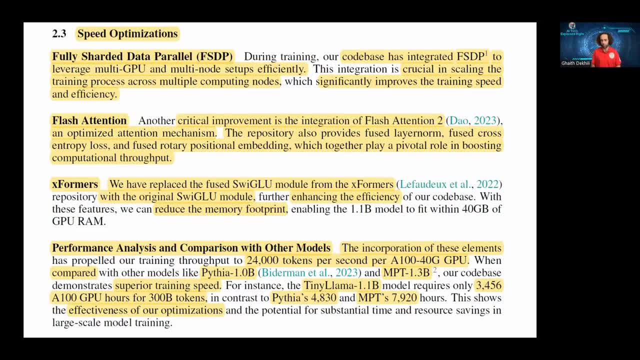 With these features, they can reduce the memory footprint, enabling the 1.1 billion model to fit within 40GB of GPU RAM. Now, authors claim that the incorporation of all these 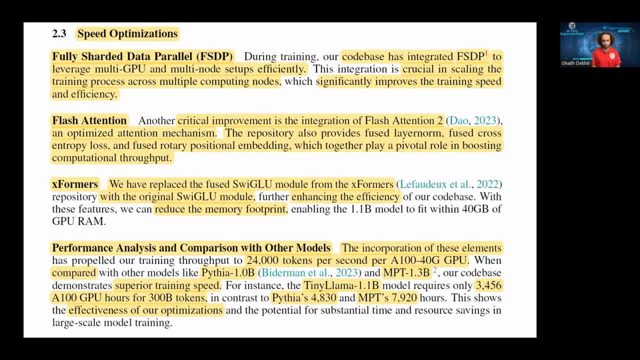 elements has propelled their training throughput to 24,000 tokens per second per a 140GB GPU, when compared with other models like Phytia 1.0 and MPT 1.0. 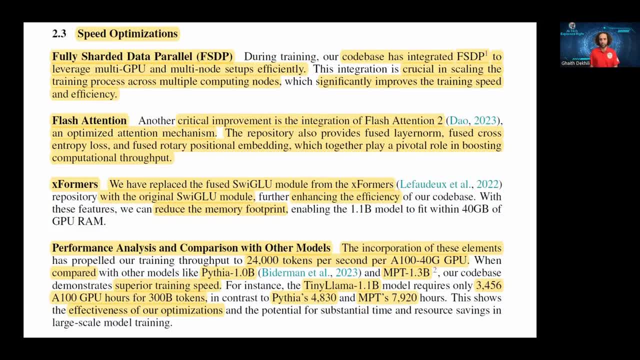 For instance, the TinyLama 1.1 billion parameters model requires only 3,456 A100 GPU hours for 300 billion tokens, compared to 4,834 Phytia and 7,924 MPT, which is a big difference. 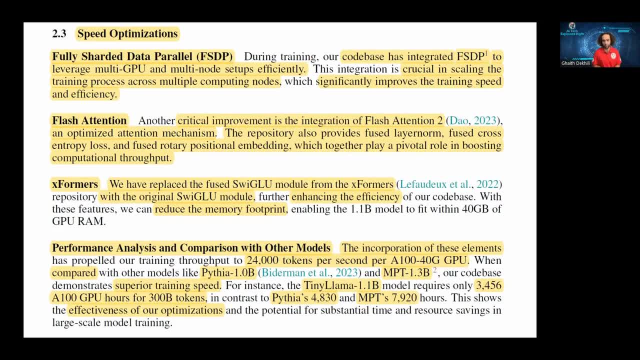 This obviously shows the effectiveness of their optimizations and performance. However, the Xformers also have the ability to optimize their own CPUs, which is a huge advantage for the Xformers. The Xformers also have the ability to optimize their own CPUs, which is a huge advantage for the Xformers. These will enable the Xformers to disable the game software 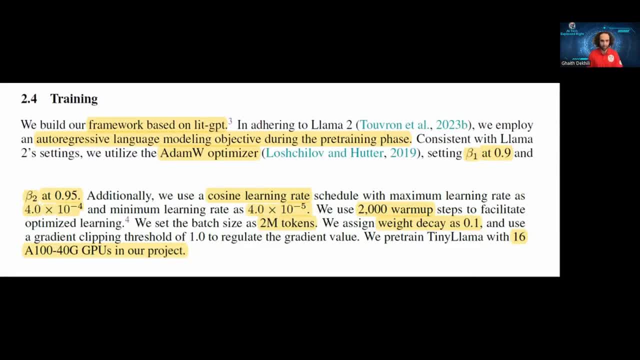 clock, which is pretty masculine inczada, to use HODL Pro in equipment or any other level ofraft. 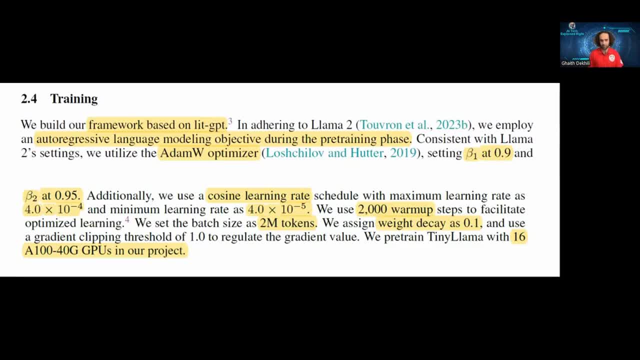 Now speaking of the devil, let's talk about training. To build their framework, authors were based ontechgpt.com. Like in Lambda included in Xformers提 http://www.phytia1.0.disk.jpg Like in Lambda too, they employ auto-progressive language-modeling objectives during the pre-training phasy. They utilized the 640켜 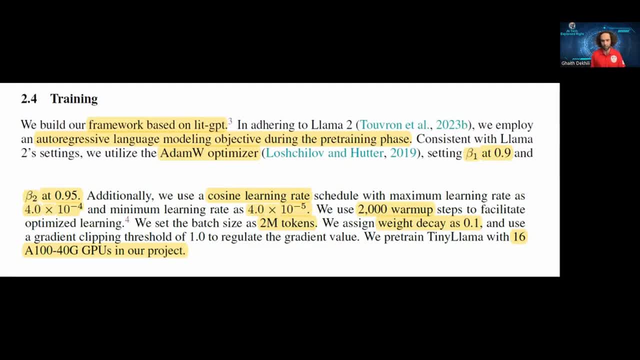 achim kalmi A villains person learning rate schedule they use 2000 warm-up steps to facilitate optimized learning they set batch size as 2 million tokens they sign weight decay as 0.1 and use gradient clipping threshold of 1.0 to regulate the gradient value and they pre-train tiny llama with 16 a 140 gig 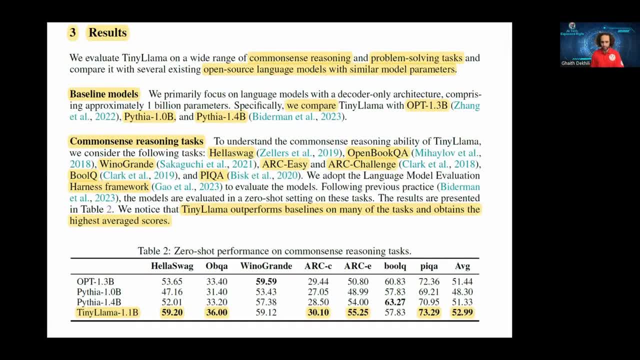 from GPUs now let's talk about results authors evaluate tiny llama on a wide range of common sense reasoning and problem solving tasks and compare it with several existing open source language models with similar model parameters they compare tiny llama with opt 1.3 billions parameters by Tia 1.0 and by Tia 1.4 billions parameters for the common sense reason test as you see in table two tiny llama outperforms the other models on six tasks out of eight and obtains the highest average scores 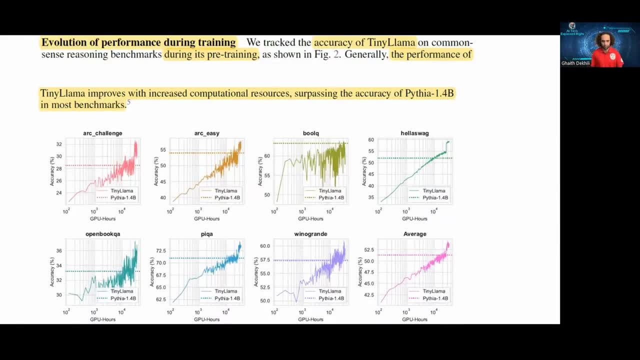 which is great authors track the accuracy of tiny llama on common sense reasoning benchmarks during its pre-training and as shown in figure two generally the performance of tiny llama improves 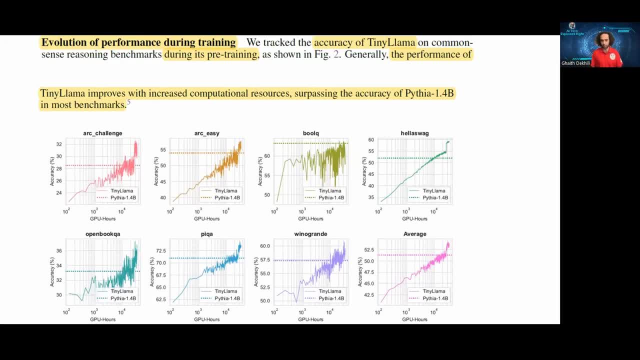 with increased computational resources surpassing the accuracy of by Tia 1.4 billion in most benchmarks tiny llama has been evaluated 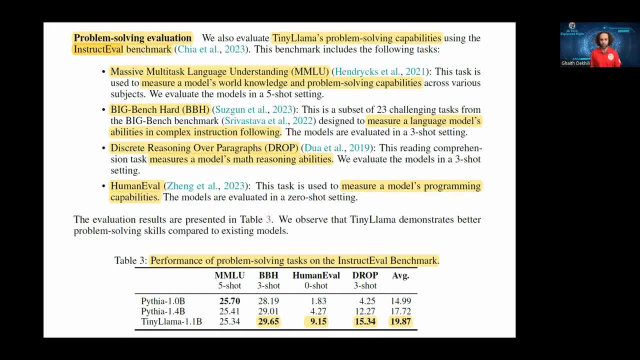 on its problem solving capabilities as well using the instruct eval benchmark which includes the mmlu to measure the word knowledge and problem solving capabilities the BBH to measure the